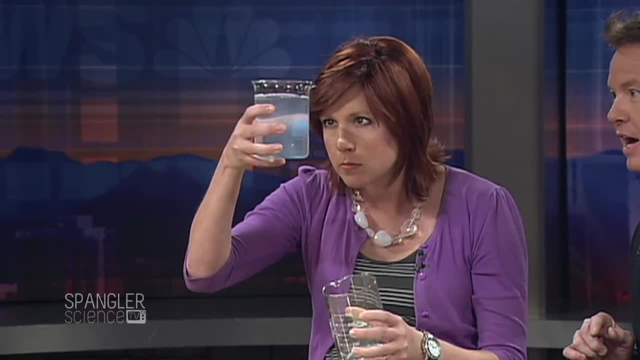 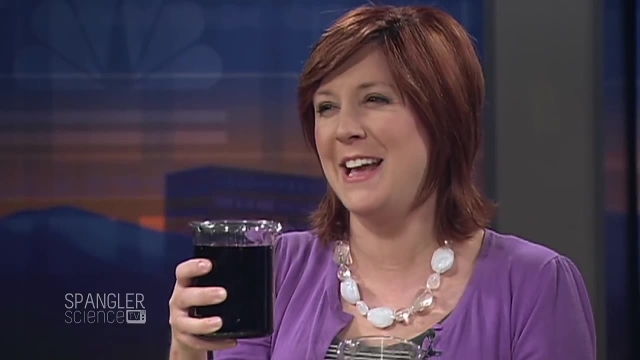 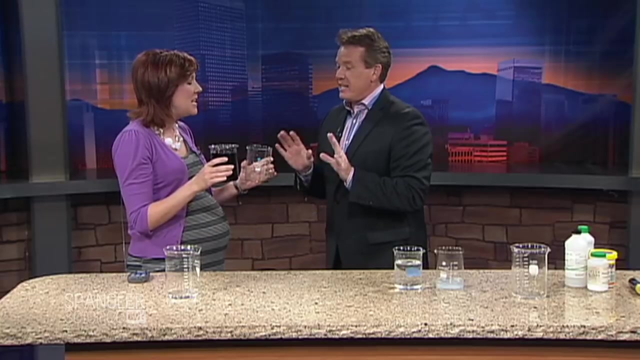 it changes color. look at it, Stare at it. Your body vibes are there. Stare, Got it. If this changes color, this is an indication that you're pregnant. Bam, Thank you. You see? that That's crazy. You are with child. No way, Because I've got the science. I know I've got the science. 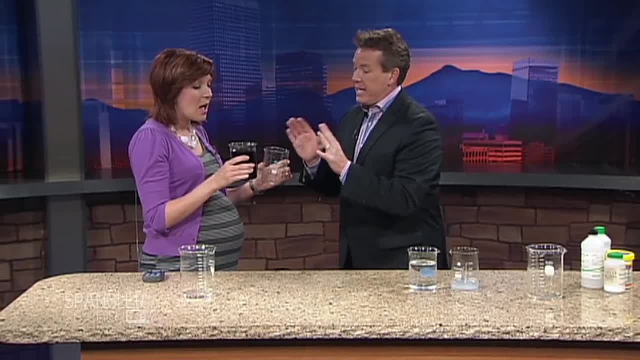 Brilliant, I know Well, thank you. And so this, this, and I can tell: watch this, See this right here. I'll hold on to this. Okay, You pour this back in here. Go pour it back in, If it goes. 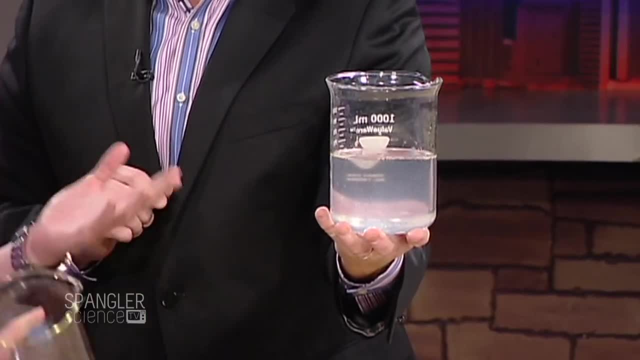 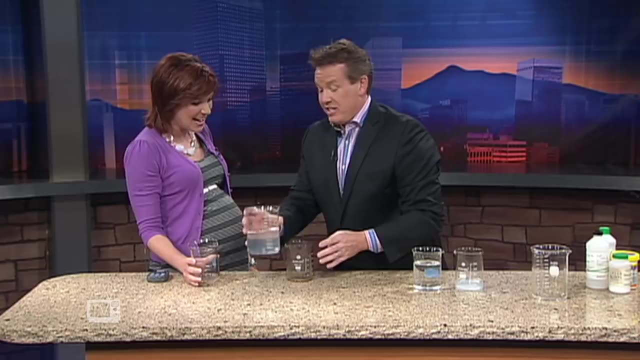 colorless. it's either a boy or a girl. Bam, What do you think about that? Boy or a girl, Right? Well, I haven't gotten that far in the book yet, but I know that it's either boy or isn't that kind of fun? So I just I broke the news here first. You are with child. 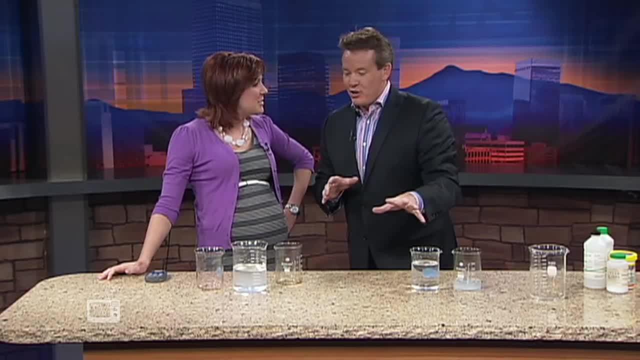 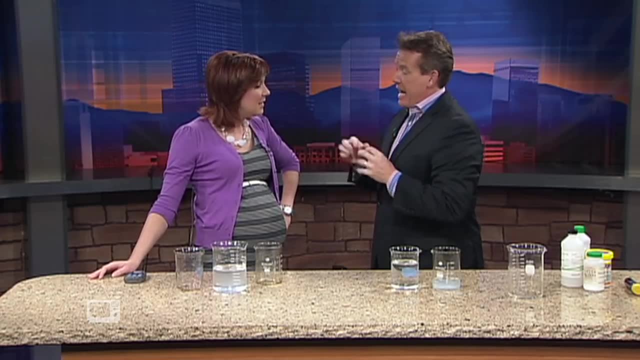 Thank you. Okay, good, Everyone Can. I can I show you. this is a classic reaction that dates back to the early 1900s, maybe late 1800s. It's called Think Inc And magicians and psychics and people. 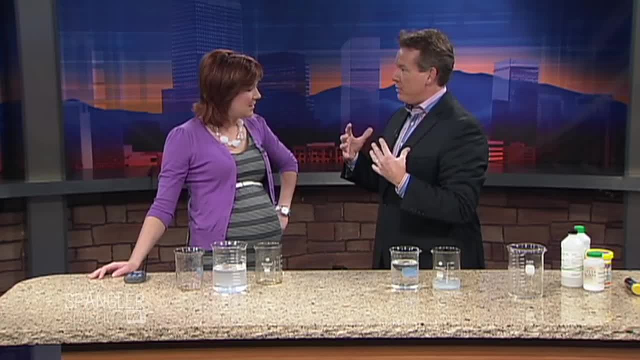 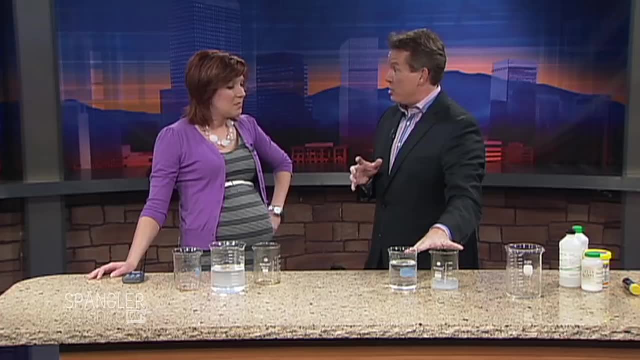 at Halloween would use this to try to cleanse somebody's body from evil thoughts, And so it's just a science reaction. but because it's delayed, it totally looks like something, And I can change the delay to two minutes, So you could really just sit there and all of a sudden you're supposed to pull the evilness out. 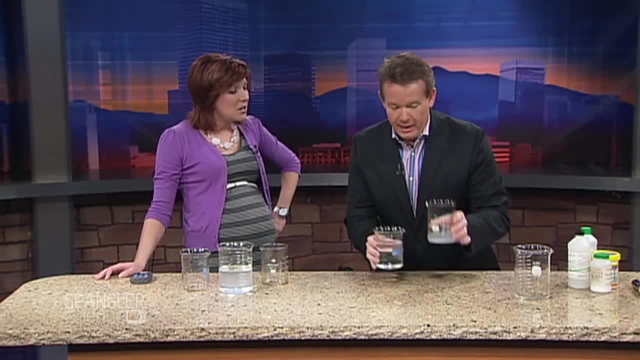 of your body, Bam, And it turns black. We're just making starch and iodine, So watch. So there's a little bit of starch in this one. here Can you see the milkiness of this Good. And then this one: 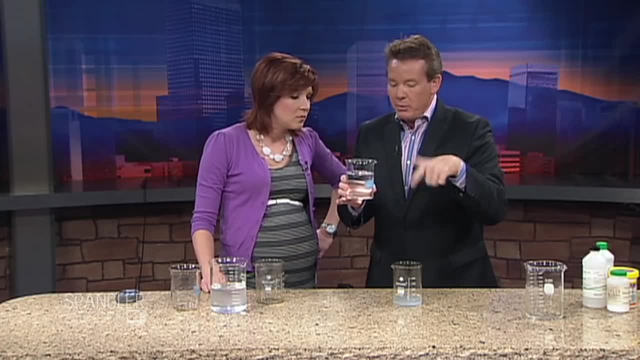 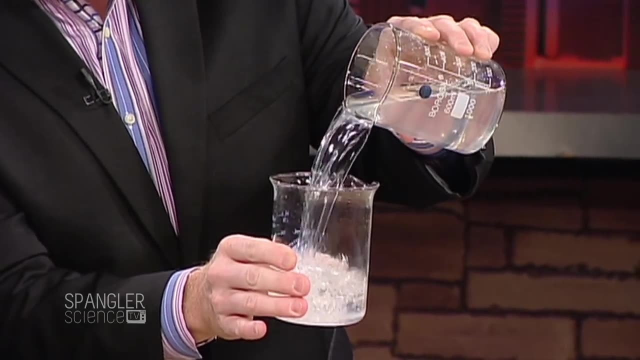 here has a complex that has some iodine in it as well, And then we set up one more process. that's a time delay. So watch as you pour them together. you literally just have molecules that are mixing together and trying to match up, And once they completely match up, that's when we get the color. 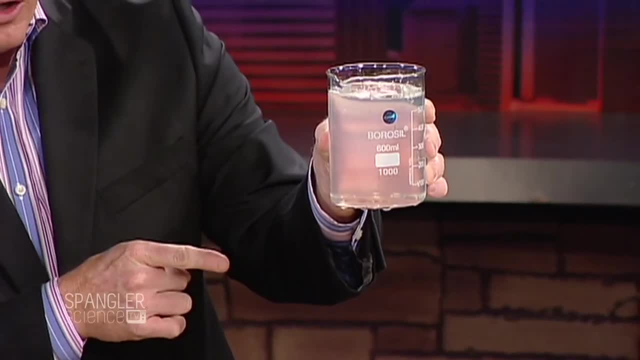 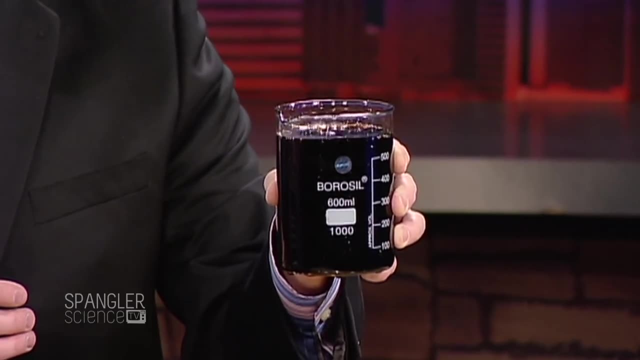 change. So you go three, two, one And as you're looking at it here, it looks like it. it looks like and you can't really tell. I've even had people drop the container because it startles them. Isn't that crazy? Yeah, That's kind of. it is nuts And 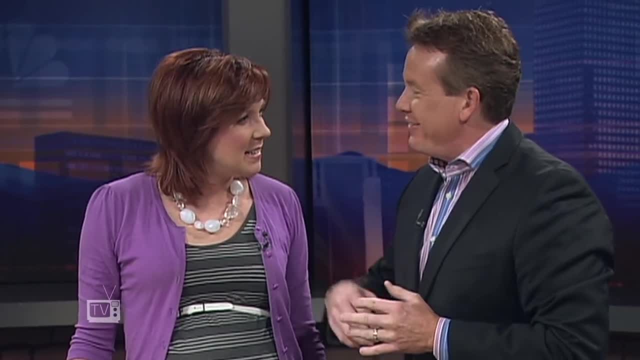 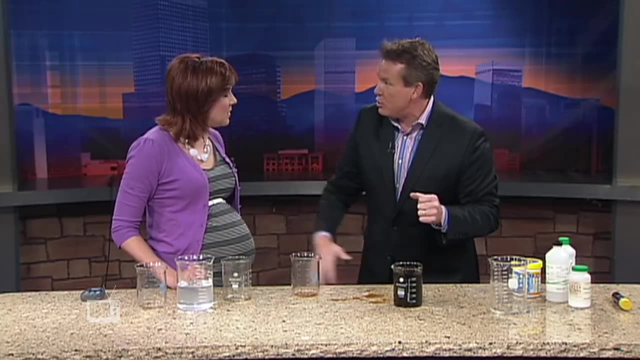 years ago there was a thing called OxyClean. Remember OxyClean? Yes, I did a commercial years ago for these people that did OxyClean, and Billy Mays had to put his hand in this big container and swirl it around and it was supposed to be coffee and ink and everything else. It was this.